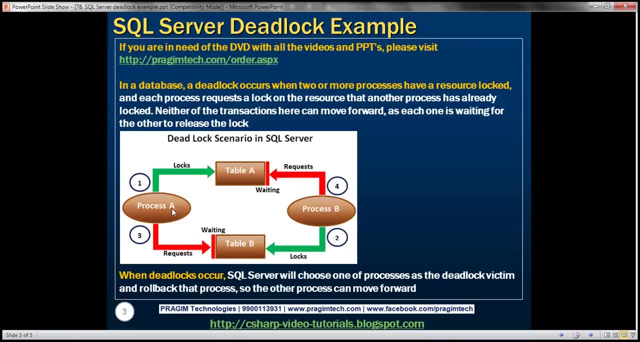 lock on table A. Similarly, process A is waiting on process B to release the lock on resource table B. So here we have a deadlock situation. When deadlocks like this occur, SQL Server will choose the deadlock victim and roll back that process so the other process can move. 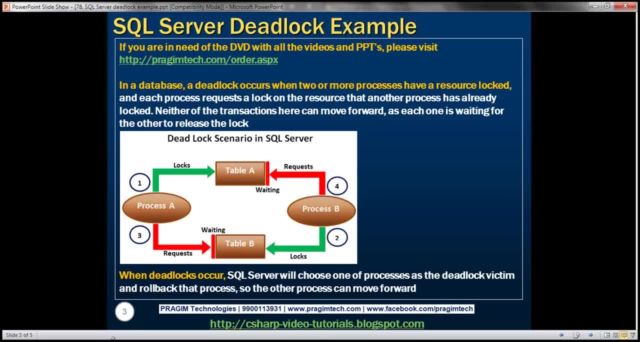 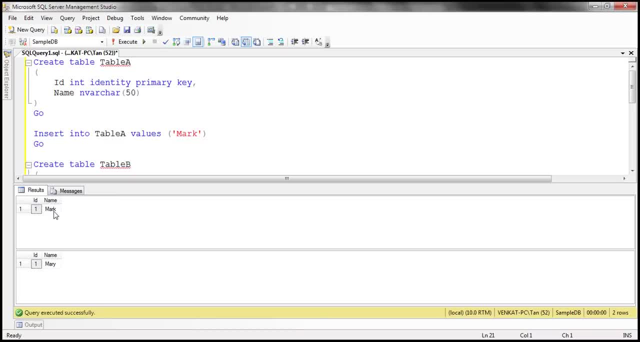 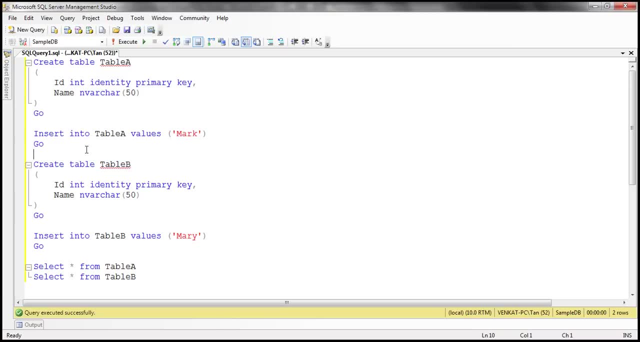 forward. let's look at this in action. I've created these two tables, table A and table B, and both the tables at the moment have caught exactly one row within each of them. and here's the SQL script: create those tables and populate them with data. I'll have the script available on my blog in case you need it. 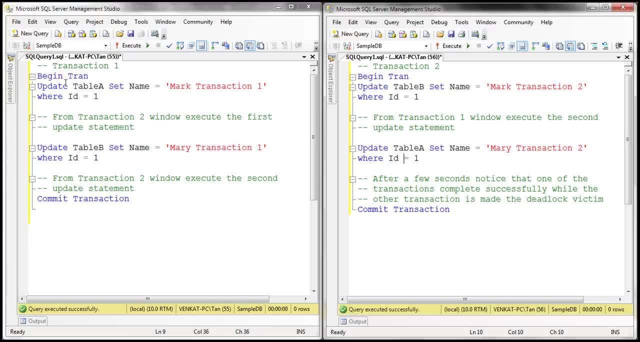 I also have two transactions here, notice. transaction one wants to update both the tables, table A and table B. transaction one is updating table A first and then table B, whereas if you look at transaction two, it's updating table B first and then table A. so let's execute part of our transaction. so transaction. 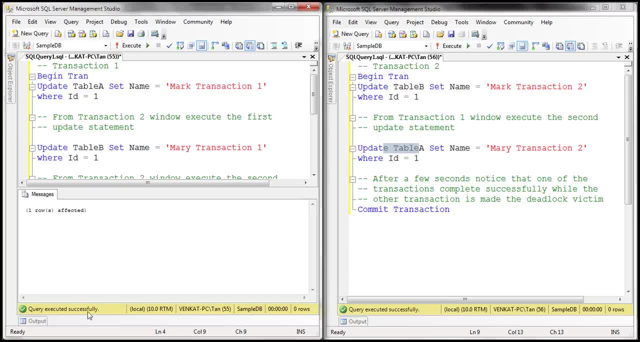 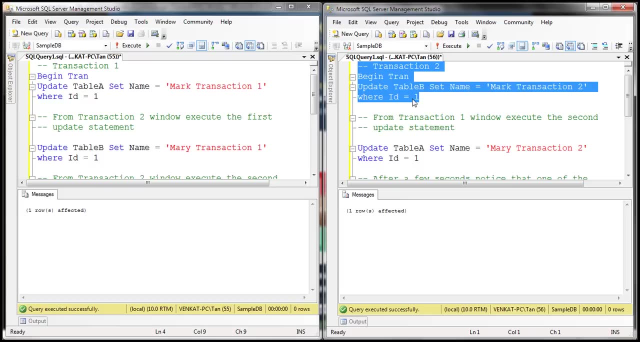 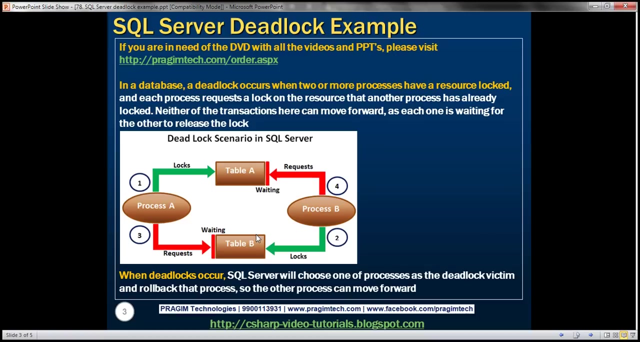 one started updating table A, so transaction one has acquired an exclusive lock on table A. now let's go ahead and execute part of our transaction two, so transaction two started updating table B. okay, so at the moment, transaction one has an exclusive lock on table A and transaction B has an exclusive lock on table B. now let's 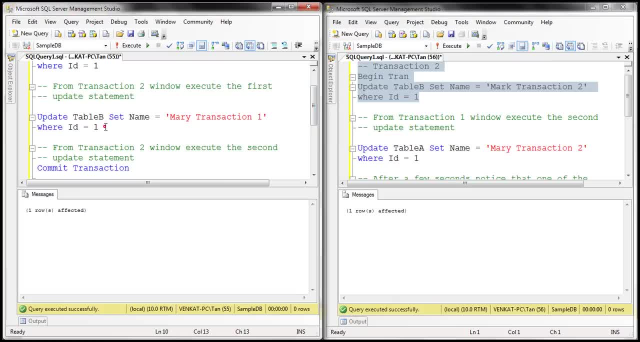 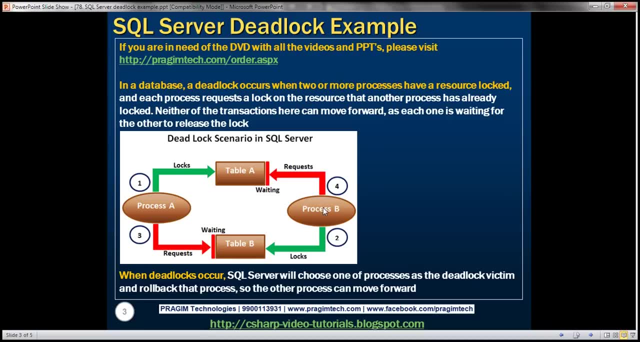 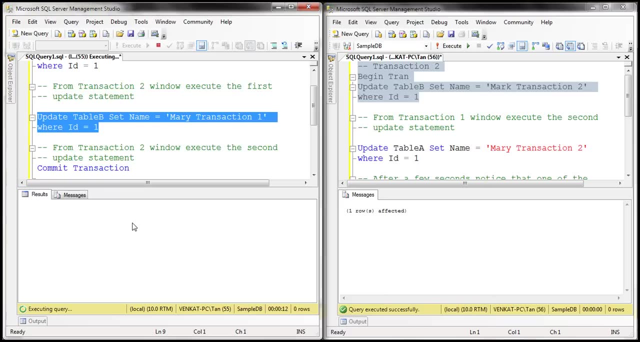 execute the second update statement in transaction one. now this will be blocked because process B, that is, our transaction two, has already blocked. you know, locked table B, so look at that. transaction two is blocked from acquiring an exclusive lock on that table. now, when we do, I mean when we 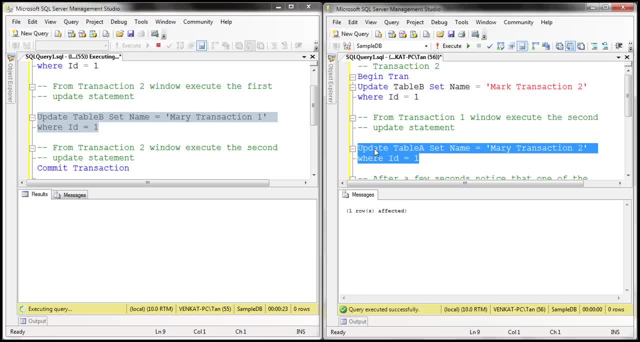 execute the second update statement that's part of our transaction two, since transaction one has already locked that resource. you know this statement, execution will be blocked. look at that: both the you know transactions are blocked now and after a few seconds. notice that transaction 2, you know, is chosen as the deadlock victim and it terminates with an.